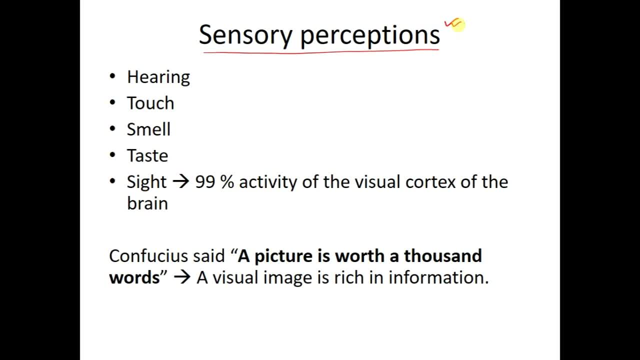 it is being processed in the human mind and again there will be, according to that there will be, some actions which will be generated by the human body. So the sensing plays an important role. So we know that there are five main senses. First one is: 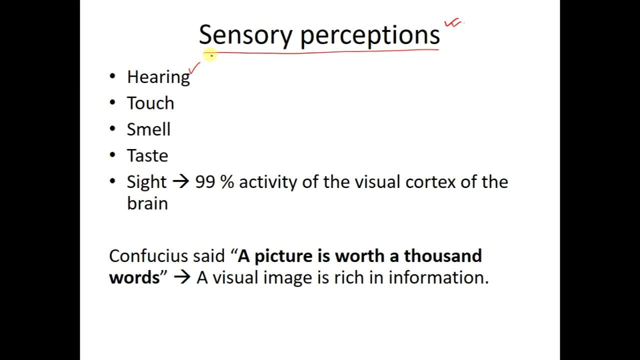 hearing, okay, It helps us to get sound information from the environment. Then touch, it helps us to interact with the environment. It helps us in estimating if someone is not able to see. someone is not able to see, then they can touch the object and by touching the 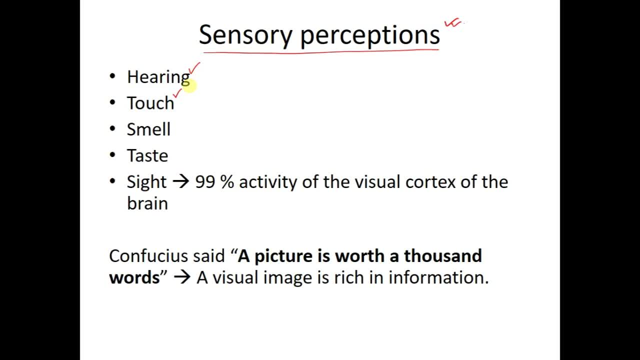 object. they can perceive the shape and size of the objects. ok, then smell it's plays an important thing. it can be a foul smell and suppose if there is any food which get it is rotten, then what happens is that you get a foul smell. ok, just by having a smell you can say, yeah, I would not take this food or this food. 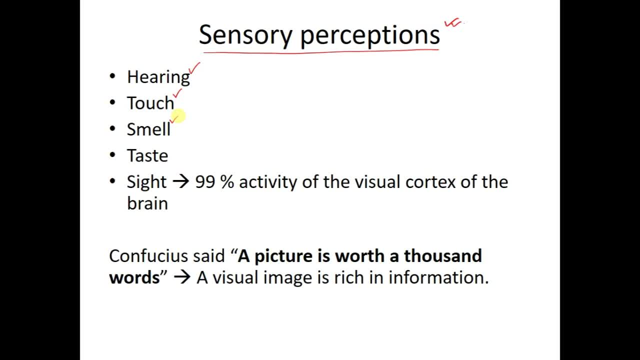 is good to me, but there is a variation in the smell perceptions, also one of the things which may not be what you call acceptable to you. it may be acceptable to me. ok, so it happens. I will give one example. in southern part of India they use smell. 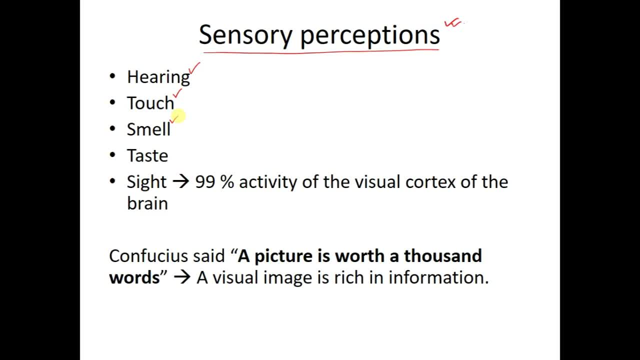 the coconut oil. so they take it in a very good manner, ok, but if you give it to the North Indians, they will not be able to eat it. ok, because there is a harsh, strong smell from the coconut oil which North Indians they have not been exposed to in their most of their lifespan. right, so going up it in a 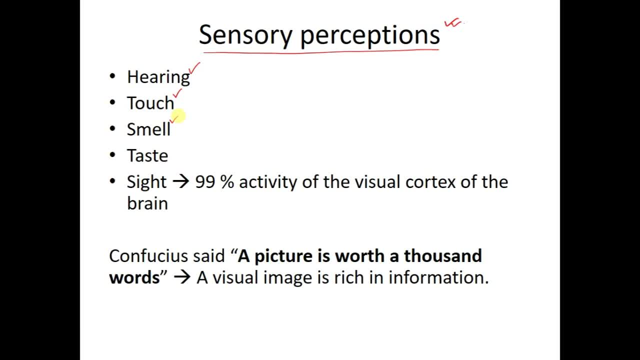 particular environment can have a different perception. ok, since it perception, then this is the same. with taste also ok, you may like a test- no- of a particular food, but I may not like that food. ok. and lastly, the site right. no, this side, it is being the. 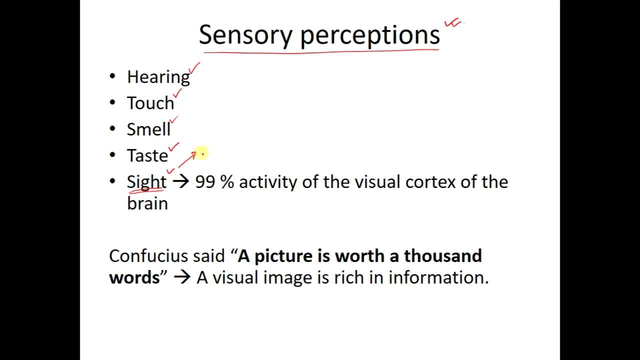 sensory organ associated with the site is- I ok now- the sense of the ability to sit down in a certain place. for Now, as per the human physiology, 99% of the activity of the visual cortex is being occupied by this side sense. So you can see, when we talk about the visual cortex, what is visual cortex? 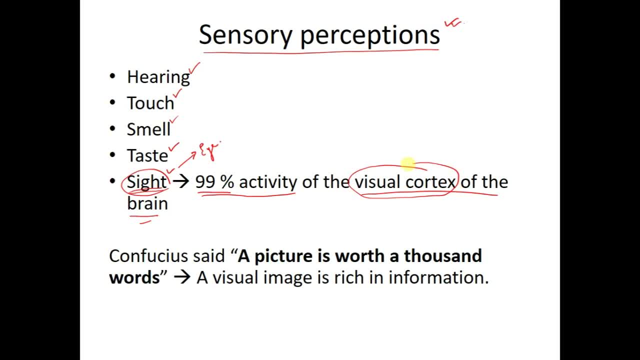 It is the part of the brain where the sense for the sight it is being perceived and processed. over there, Our brain is basically a processor and our eye, it is basically a sensor. It is having rods and cones And, based upon the excitation of the rods and the cones cells, those signals are being transmitted to the brain, to the visual cortex. 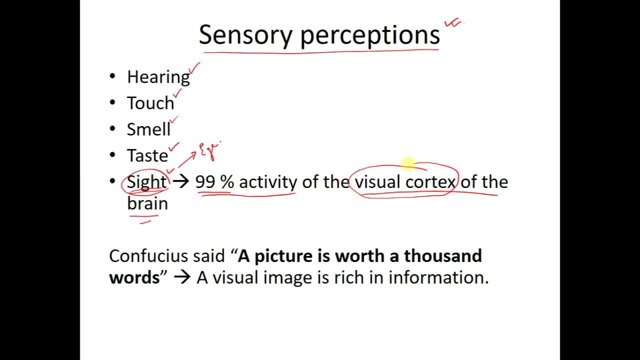 And in the visual cortex this information is being processed. Now, if you consider the thing when we wake up, since that time till we go to the bed, our eyes are giving us continuous information and because of this reason, what happens is that we are, I am able to perceive one person from the other, a boy from a girl. then again, the color information comes over here so I can differentiate the colors. so there are so many things so, because of which our life has become quite easier. without sight, our life is very- it would have been very difficult. 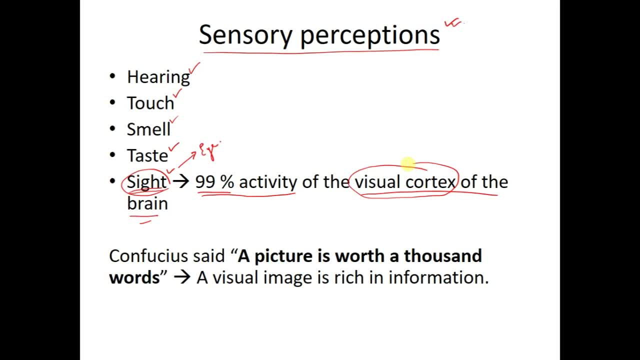 Now, essentially, what does this mean? what do you call tough right? So, accordingly Confucius, he is one of the philosophers. he said that a picture is worth a thousand words. Suppose I have to describe one of you, and if I tell your colleague to describe you, how will he describe? 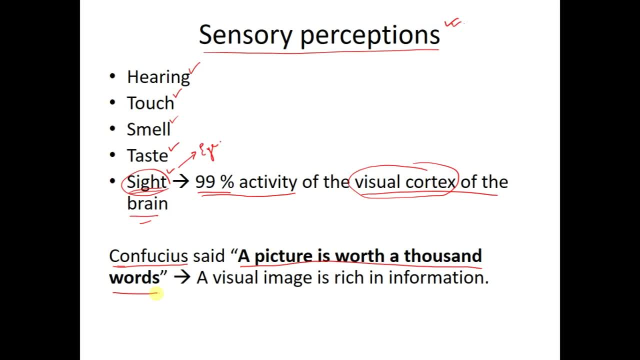 Why What? Give me a question, Give me a question. Give me a question. I say: don't draw the picture. you describe the person in words. is it possible to describe everything? because you will need a lot of wordings to put into a sensible know what. 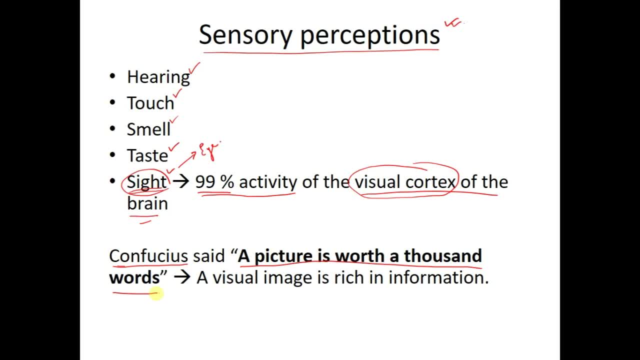 you call sensible writing, which can particularly define a particular person, okay, but still then another person may not understand the whole thing, he may not perceive the whole stuff, what has been written, okay. but on the other hand, if I give you a picture and then I tell the person you describe this person, then it becomes much easier then making the other. 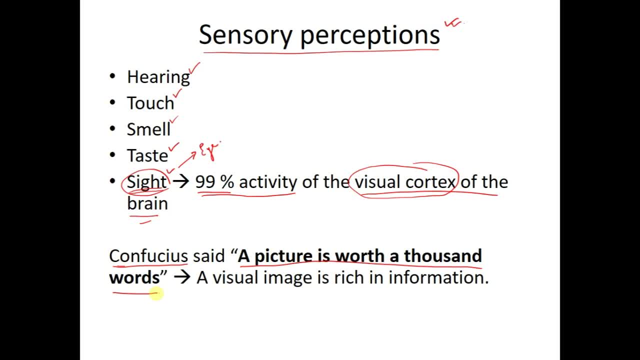 person understand, it becomes quite easier. okay say, for example, I want to design a helicopter. now that design, if I try to explain you verbally or in a written format, it will be very difficult for me to describe the whole thing. but if I draw it and then mark that this is, this should be the length of the vertical blade of the helicopter, this should: 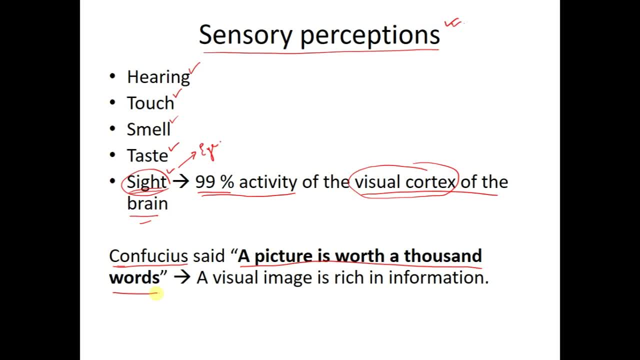 be the length of the tail of the helicopter. it should be the height of the helicopter. then it becomes much more easier. It is easier for another person to understand and recreate the same thing. okay, and this would be quite useful while you are designing any devices. if you see the development of 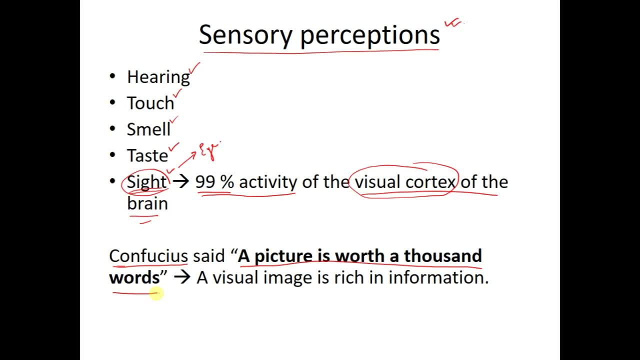 the images. it's an important thing in the next two classes to have a feeling what image processing, how image processing can help us in various medical applications. we will be looking into the projects being done by Ankit- Thank you- and Deepak, in the next two classes so that you get a feel, and then from the next week onwards we will start the main lectures. okay, so those will be the application parts. so, because if you see the thing at the start of the course, then you will be able to correlate the stuff, what they are doing okay and how you can apply those algorithms over there. so that would be my primary, what you call. 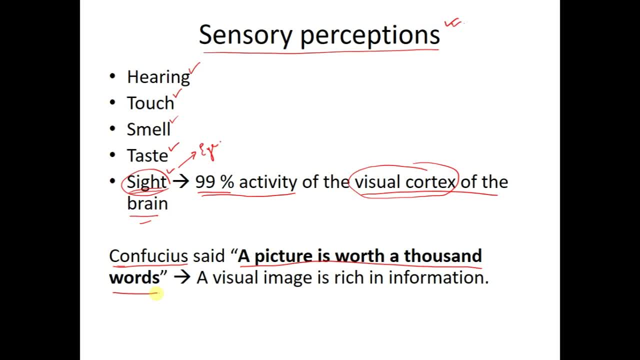 primary concern, right? so, as i told you, a visual image, it is rich in information. a single image it can give you a lot of information, whereas if you write 10 pages of your, of your, of a question, it might not be as informative as your images. so, from here, 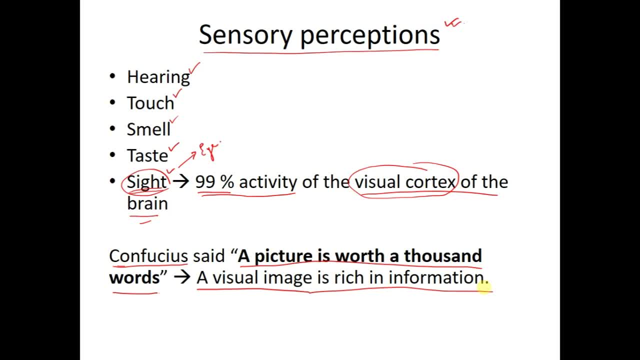 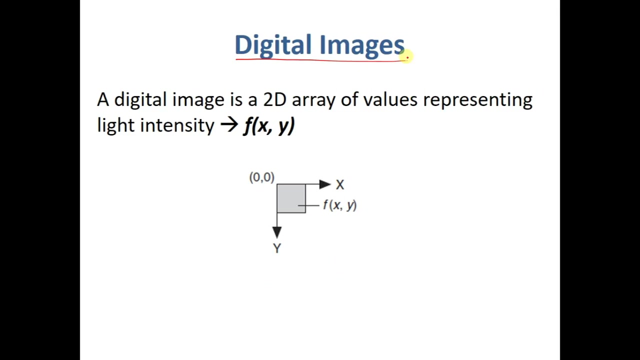 I would like to say, while you are writing the questions and answering the questions, for the image processing, this thing, try to put as many figures as possible, okay, and if it is a numerical, that's a separate thing. now, coming to the digital images, what are digital images? if you see the 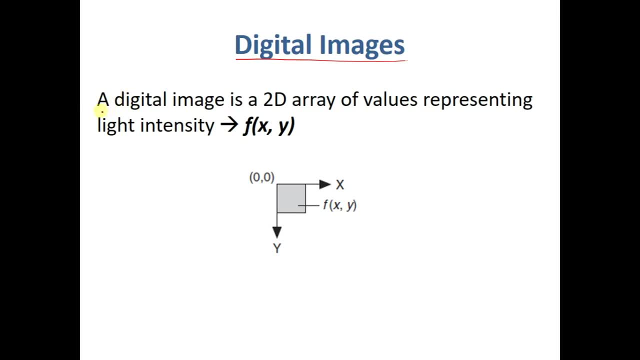 definition of a digital image. you can see that the definition of a digital image is the definition of a digital image. you can see that the definition of a digital image- it is regarded as a digital image- is a 2d array of values. it is a 2d array of. 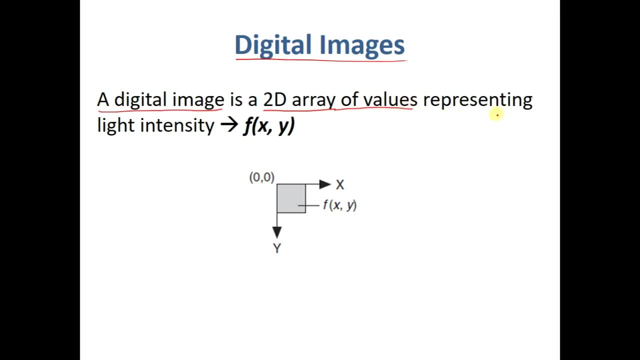 values that represent light intensity. so what are these values? these values are light intensity. I would like to again remind you, which I have already discussed in the previous classes: image processing means grayscale image processing, where we are having only one plane. if we are talking about image processing for the color images, then I 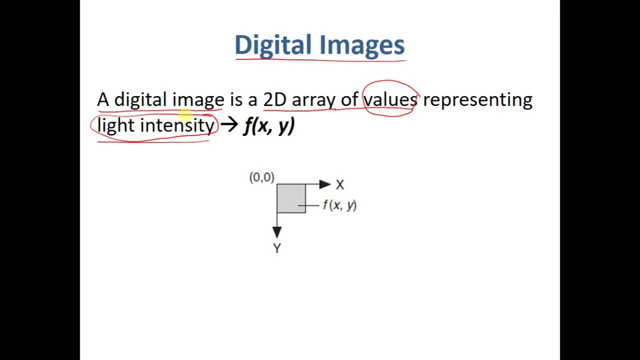 would call it as color image processing. okay, so image processing as a whole. it was, as I previously also told you, that image processing was previously developed for the grayscale images. okay, so please be reminded. now a digital image. we have seen that it is a 2d array. 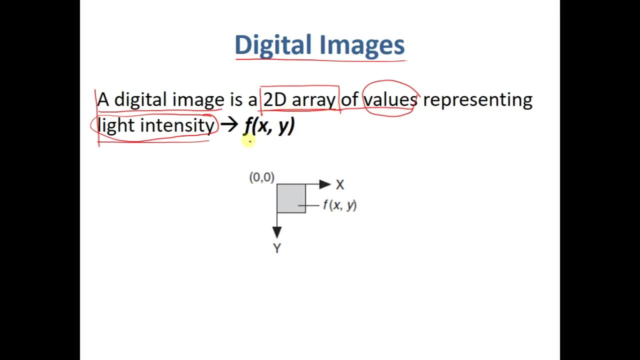 okay, and it is represented with a function f of x, y, okay, 2d array means it will be a 2d matrix like thing, not exactly matrix, but we can represent it, represent the images as the matrix. So suppose this is an image. this is a digital image. 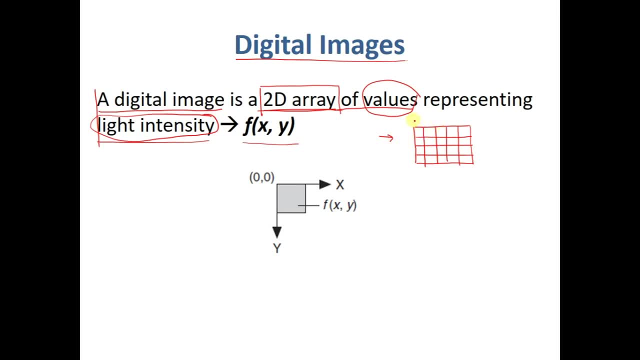 suppose. So this is x axis and this horizontal part is y axis, and here we have got some boxes. Now, these boxes, they are regarded as pixels. Usually, pixels are square in nature, but it depends. Square is the most common pixels, square pixels are the most common. 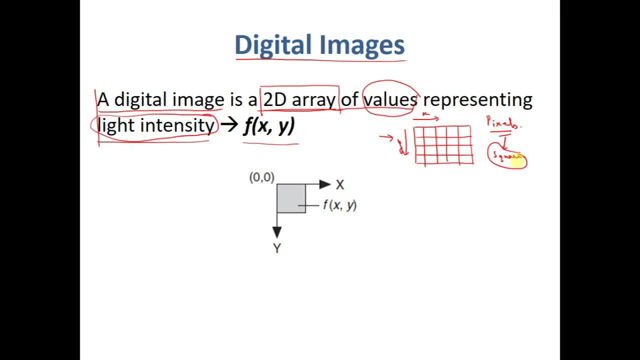 pixels which are used and which have been adapted by most of the industries. but pixels can be rectangular, it can be circular, So it depends on how the image acquisition system has been designed. but in general, pixels are square in nature. So, if you see, what I said is that a digital image is a 2D array. 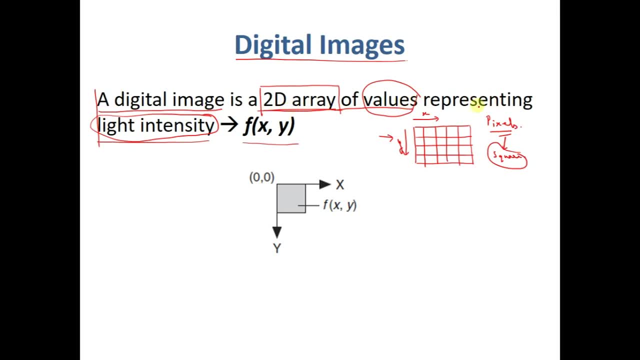 of values representing light intensities. So 2D array of values. So these pixel values, these pixels basically houses some values. This blue marks these are basically some values. So what are these values? These values are light intensity for a 8 bit image. the values may vary from. 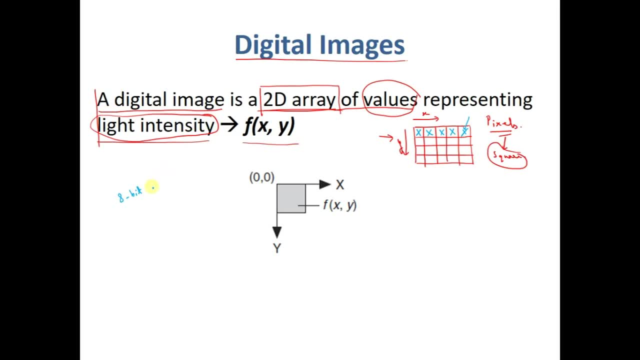 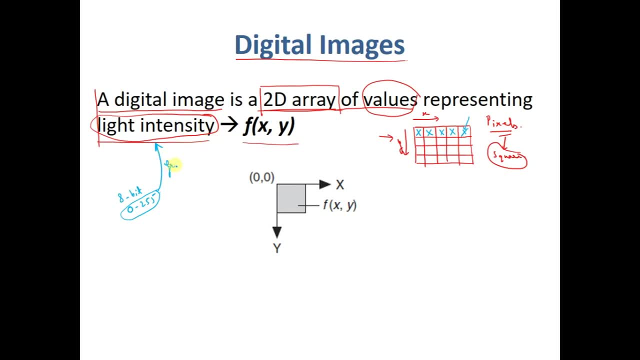 level values. you get my point. why gray level values? because I am talking about only light intensity. light intensity is white, complete dark to complete white. in between you will be having shades of gray. usually most of the images, especially the medical images, they are grayscale images. okay, now, if you see, 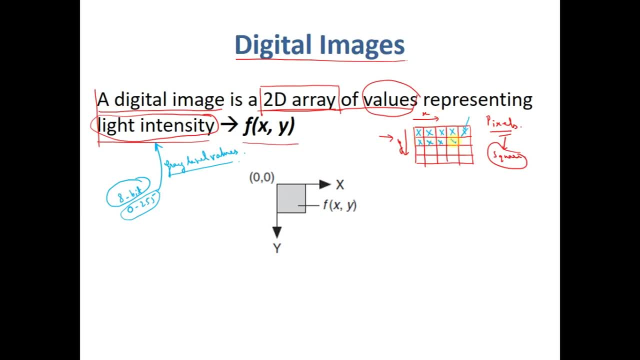 these are a series of values in the digital images we are having this series of values. okay, now they can be represented as rows, as columns, similar to a 2d matrix, and hence, when we talk about processing, image processing, we call it matrix operations. so, whatever the matrix operations. 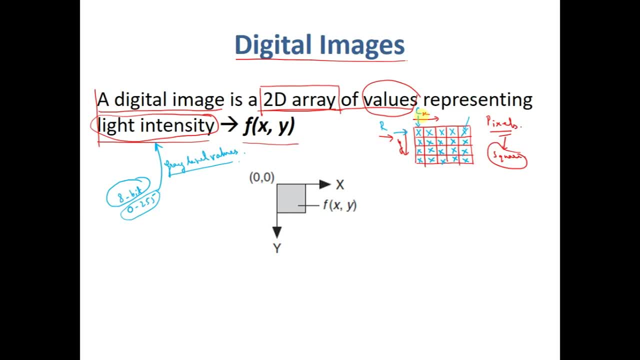 are there. those are also applicable over here also. okay, but there is a certain difference. while we are doing the matrix operation in the digital image that I will come later on. okay, now, over here, what is happening? if you are having this points, then we can pinpoint the location of the intensity values. okay, now, this starting point we are going to be. 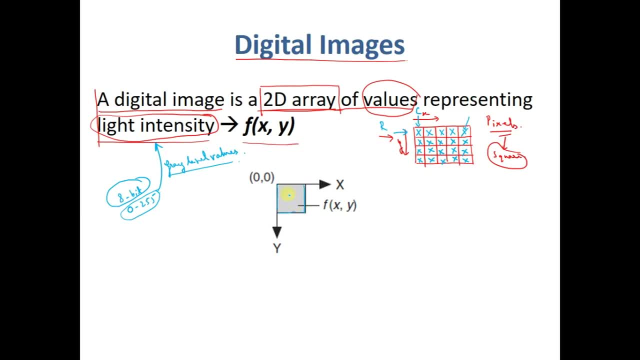 looking at the starting box, which is basically the left most top pixel, okay, that means this pixel which has been highlighted in green. okay, this pixel, the coordinate of this pixel is 0, 0. put it as we usually name it, as 0, 0 pixel. okay, but in many books you will find that 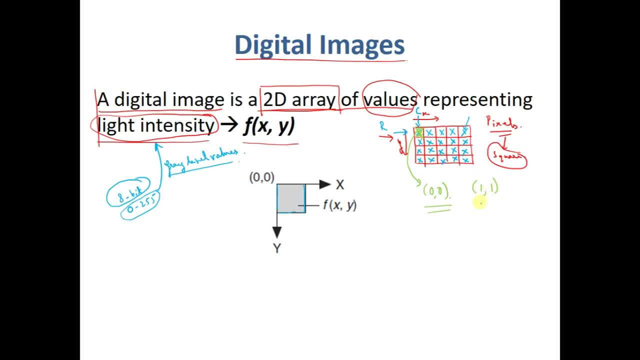 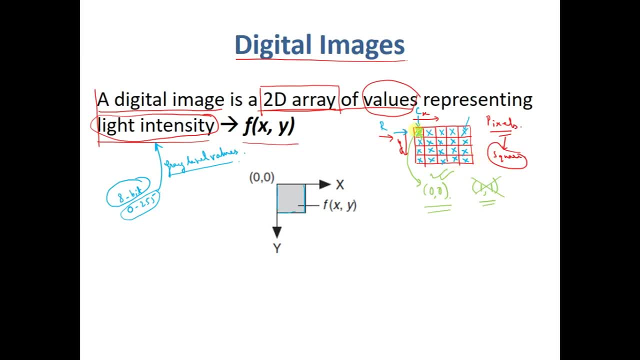 0 0, 1, 0, 0, 0, 0.. coordinate system. So this is 0, 0, 0, 1, 0, 2, this is 0, 1, this is 0, 2, and so on. 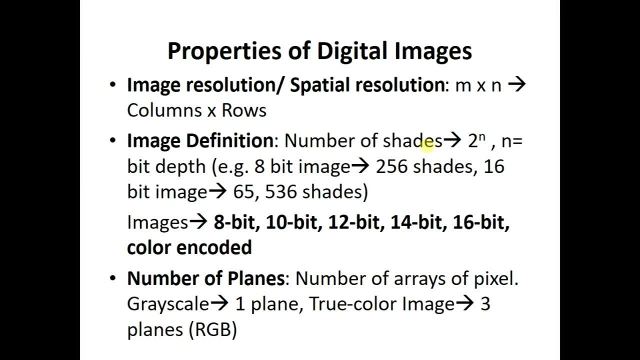 Any doubt, No Good. Now, coming to the properties of the digital images. What are the different properties of a digital images? First one is image resolution, which is also regarded as spatial resolution. Now, it is given by the multiplication columns, by rows, Columns. 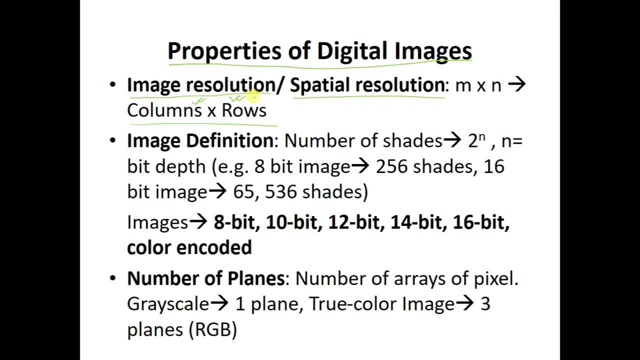 and rows. What is the resolution of this image? The resolution of the image is whatever will be the number of columns multiplied by whatever will be the number of the rows. Then, coming to image resolution, Next definition: It says how many numbers of shades are there, And it is being given. 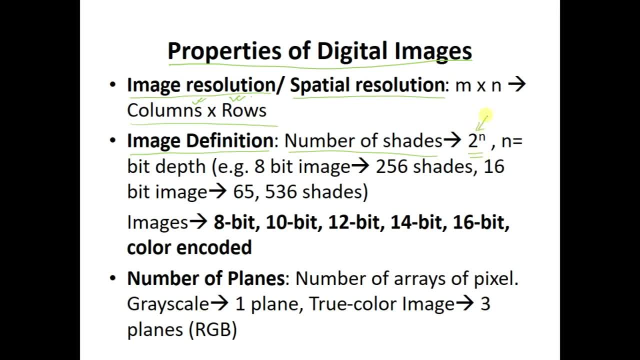 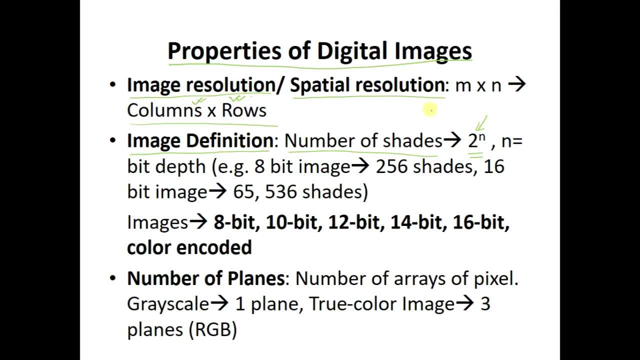 can be can be can be in the digital signals. your amplitude values can have values in 2 to the power n values, where n is the bit, where n is the bit depth. So for an 8 bit 1D signal there would have been 256 number of values: 0,, 1,, 2,, 3,, 4 or 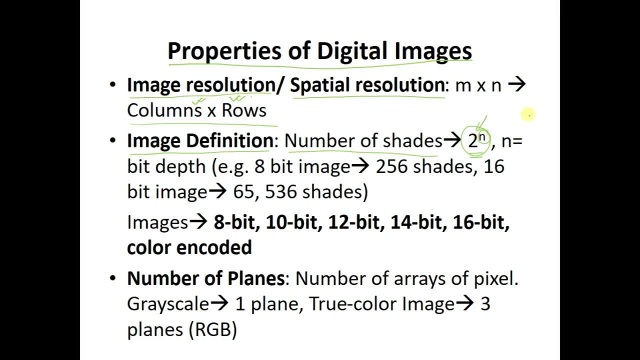 something like that Right In image. an 8-bit image can have 256 shades- 256 shades In signals. we are having amplitudes, Whereas in image we are having shades. Accordingly, 16-bit images image, it can have 65,536 shades. Further images can also be color encoded in 8-bit, 10-bit, 12-bit, 14-bit and 16-bit. 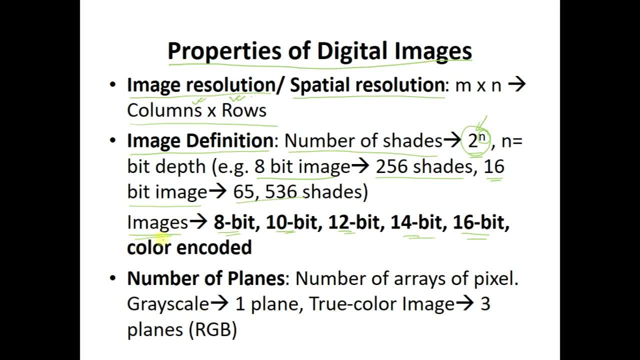 Or the grayscale image. So there is color encoding. This can be done in all these fashions, But grayscale images also. they can have all these bit images But, as I said, for medical imaging purposes 8-bit images provides us sufficient number of this. 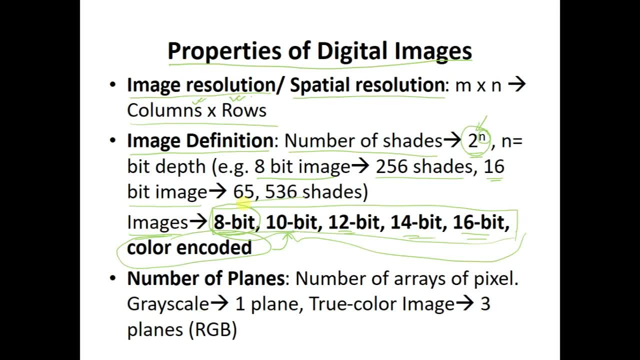 Shades which can help us in understanding the human physiology for clinical relevance. Hence, there is no need to go for the higher bit images. Why? Because when we go for the higher bit images, that means you need a higher, higher storage to store those data. That means the size of the file will be more. So why? 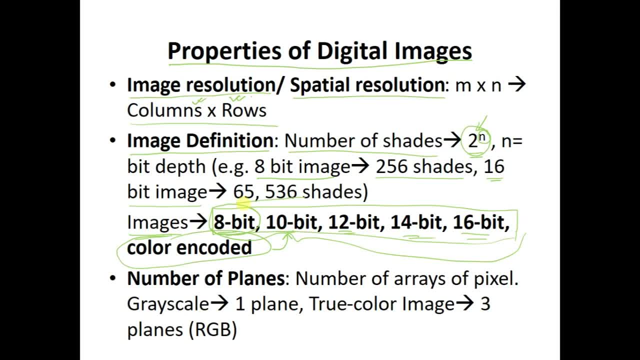 you want to go for losing of storage, Because you are getting the clinically relevant information through the 8 bit image itself. Then, coming to the number of planes, So what it says It is the number of arrays of pixels. In a greyscale image. we have only one plane. 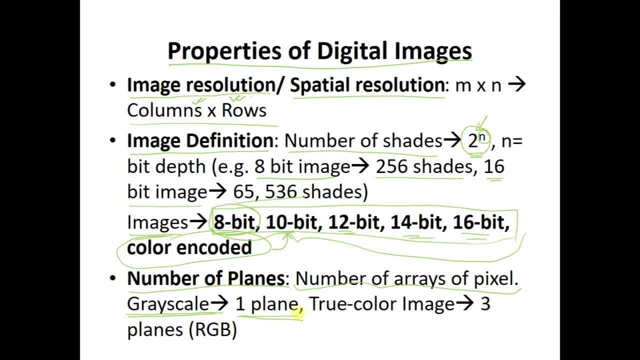 It is just the light intensity value. But if it is a color image, say for example, there is a color model, RGB model, which is quite frequently used. So you also might be knowing that RGB model is there. So our computer screens and most of the TVs and all these things, they look for this RGB. 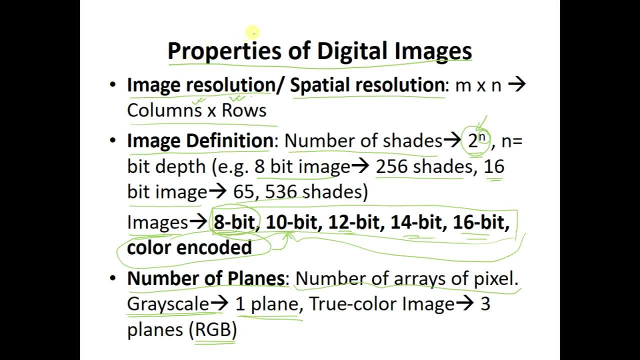 model, They go for RGB model. Now, over here, even the LED TVs or LCD TVs, they are having this what you call the RGB model. They apply the RGB model. So what it says is that it says the anytime you put the LED in to a color, it will display the코. 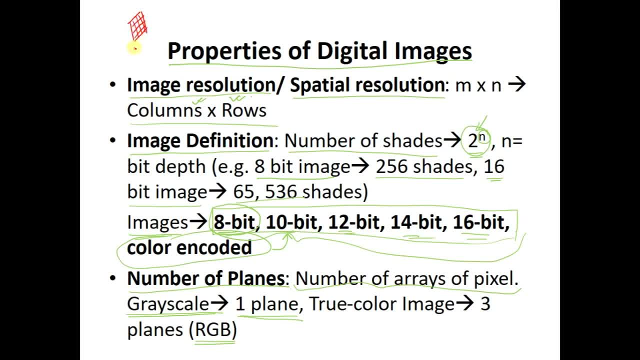 im建ие LED activity like this. You will receive the test load of all the LEDs in the area. You will also be getting that control room of the Nobubрист to look for annoying objects. You will also the LED everywhere. For each color image, you will be having a red plane, green plane. Therefore, from the color image that you are adding, you will see different gains. When you check the color of the green plane green player, look into the red element. You will get a more blue圓 green color For each image of the AMD powder hive. we have a red memang For match of ends of탁. this is the sign of радox俺. 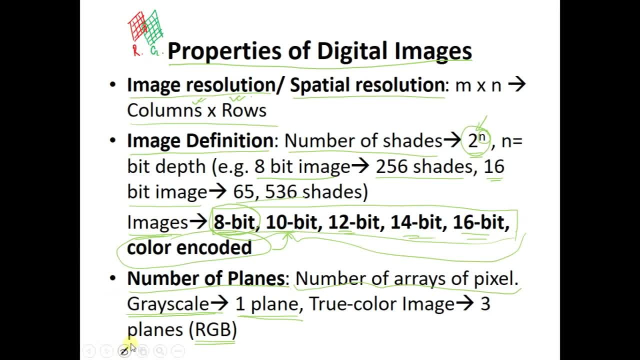 Red. nod, get into red, a better colour, Right, let us see, we know how it is. All right, Green plane And a blue plane. Okay, Now the number of the pixels. they are same in all these things. That means the image resolution for all R, G and B planes are same. 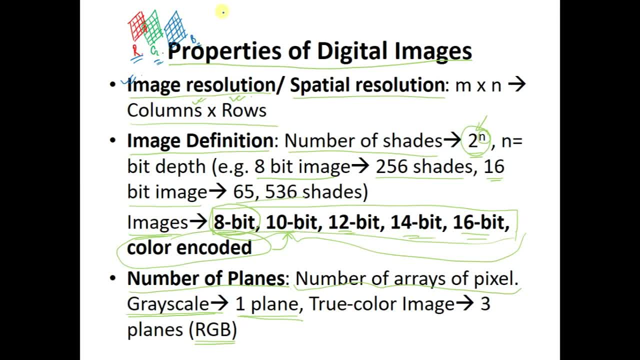 Okay, Now what they do is that? what it does is that it combines the information from all these three planes in a pixel to pixel manner- Okay, In a pixel to pixel manner, to generate an output which is having color information, or in other words, true color information. Okay, So why this three planes? It is because you can. these are the primary colors and you can synthesize any color, just. 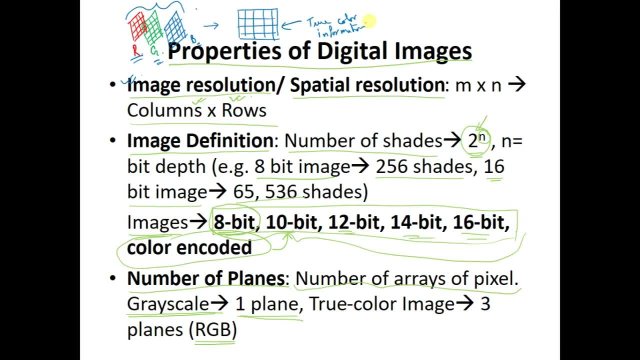 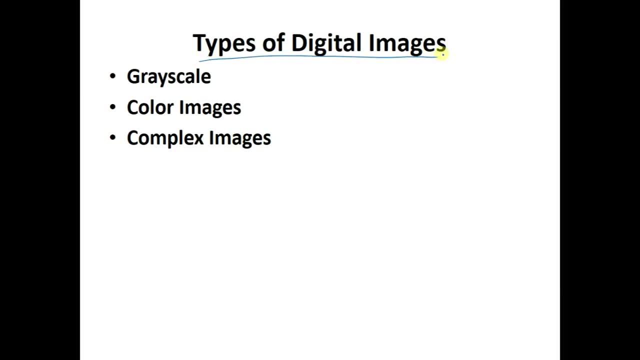 by mixing the various shades of red, green and blue. Various shades of red, green and blue. Okay, Now types of digital images: grayscale images. I have already told There will be one plane, Color images. it should have three planes, Okay. 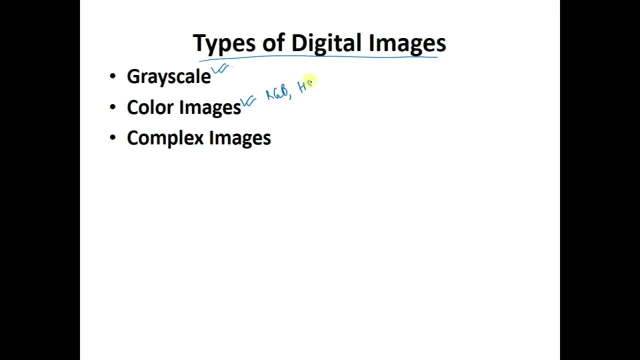 Whether you talk about RGB or HSI model- Okay- Or CMY model, Whatever model, you are talking about all the color planes. they have three planes, Okay. Then, lastly, complex images. So can anyone tell me what are these complex images? 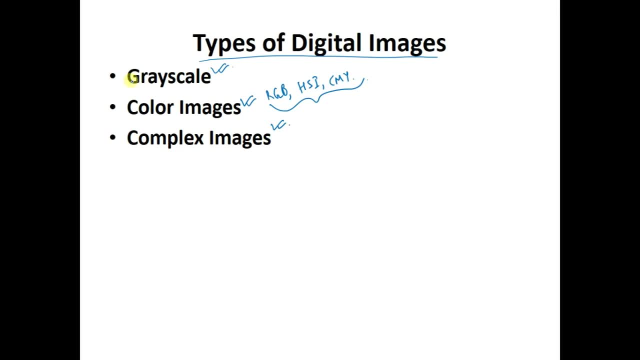 When you talk about these grayscale images, these are in the decimal domain. Okay, When you do Fourier transform, what I said in the introductory class, Fourier transform of an image is also an image, But that image contains values which are complex numbers. 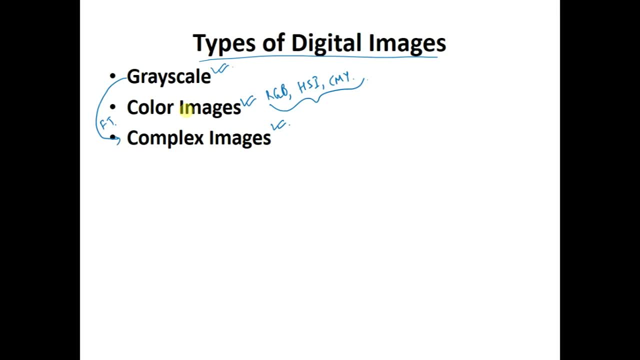 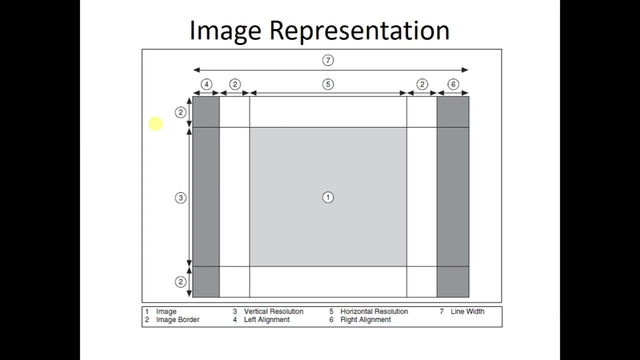 Which are complex numbers. Right, That's why they are those images. they are regarded as complex images. Okay, Now coming to the representation of an image and how it differs from the matrix. When we talk about matrix, we have only the numbers. 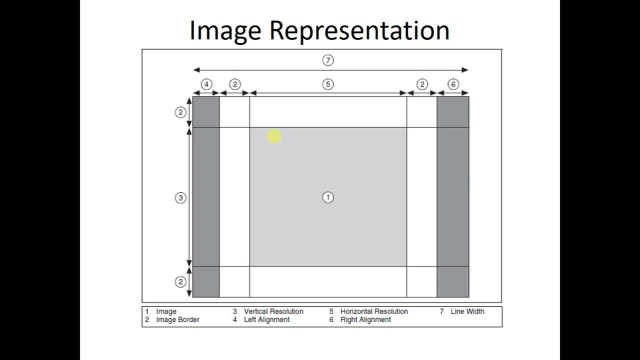 which are there present, but image is not the same. okay, if you look over here, image is this number one part. what is that? this is your image. this area, this great shaded area. this is the image, okay, and this image it has been taking from National Instruments, this, they are having one manual. okay, for image. 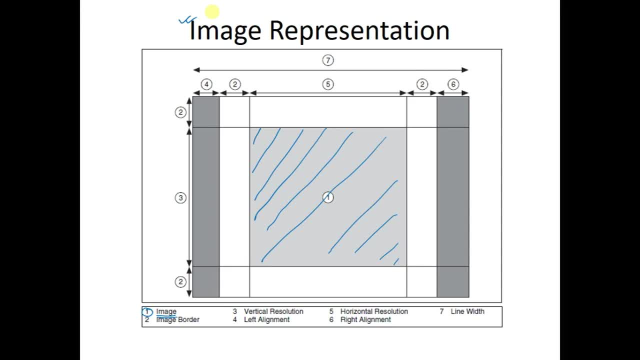 processing manual is there for vision machine vision applications for vision, which is regarded as vision assistant. okay, so this image has been taken. most of the images of this lecture has been taken from there, so we are having this as the image, but when we try to possess it, we cannot confine ourselves within this area. we 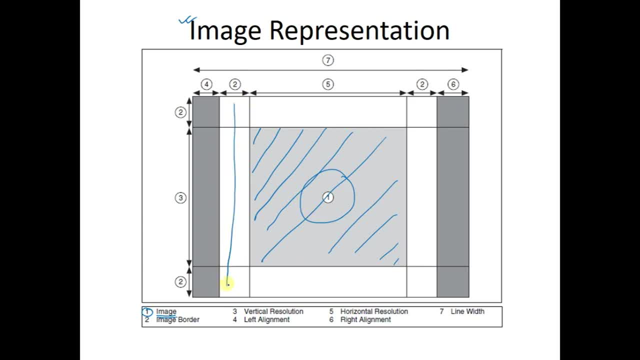 need borders, this white area. they are called borders, so to: this is the image border. okay, this is a image border. okay, then 3, this is vertical resolution. that means the number of rows. okay, similarly, documentary. 5 is the horizontal resolution. that is the then image resolution number of Bryden. 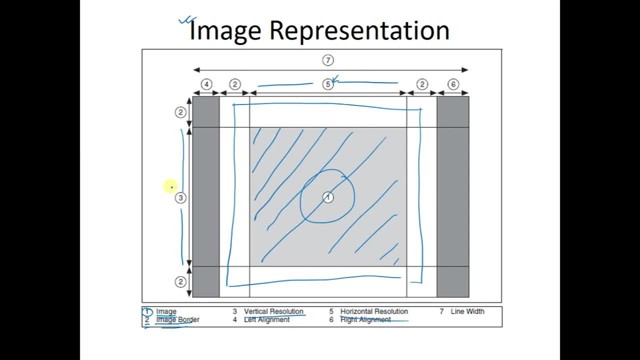 Wolfson's UM code完. five and number of three. that will be your image resolution. we have already talked right. then seven is the line width, this total width of this thing, and what is this? four and six? these are left alignment and right alignment. this left and right alignment. these are not needed in most of the 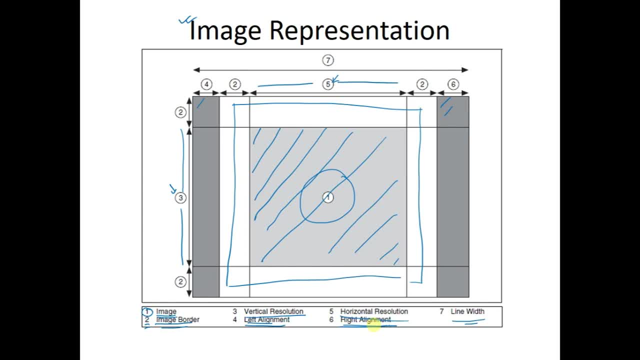 cases. but when you go for the bar coding, the alignment becomes an important part. so you have to align the image and then you can. you have to go for the machine reading applications, okay, but for normal this processing, we basically need the image component and the order component. and why? 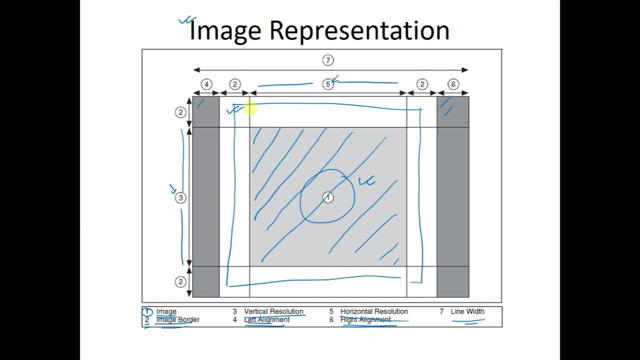 why do you remember your signal processing class? how do you implement filters in the time domain, filters in the time domain, digital, digital signals? okay, how does the vos 1ics work? you apply convolution, so you are having, say, one number, two, verticalco mówią three, two, one, something, say if this is the signal. 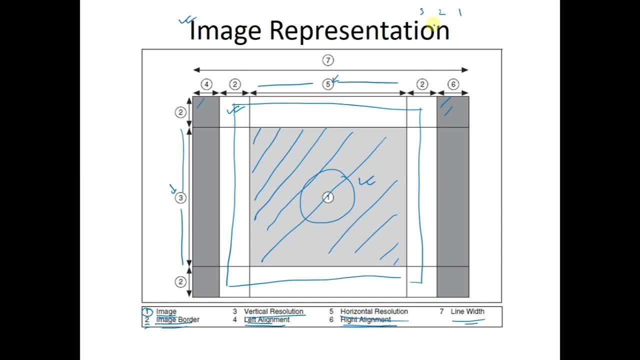 and if there is another"primary number is value one, one, one one is there, okay. so what you are doing? because these two ones, they are not what do you call and they are not active. it is working and so you just have to communicate here so youie save the noise. notice, if you keep applying resolution, so you apply convolution, so you are having, say, one number three, two, one, something, say, if this is the signal and if there is another average, what you call repair number, number three, one, one will be there. so 11 or one is there, okay, so what you are doing. so what do you are doing? these two ones, they are not what you call and they are not a 베 was after 100. 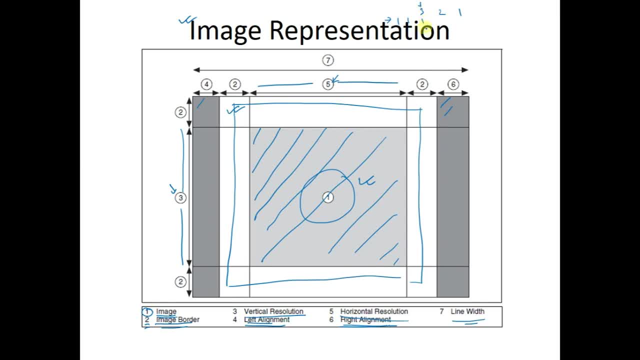 what you call. they are not aligned with the zero of the signal and this thing. they are outside this range. so what we do, we do zero padding. what is that? it is in the one domain. you are doing the padding in one direction. similarly, when we slide this thing, we need zero padding. 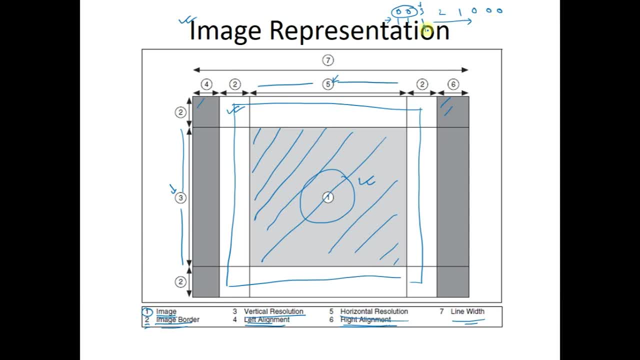 at the right hand side, also right. yes, many blank faces are you getting. have you understood or not understood? i have asked a simple question: have you understood or not understood? either you have understood or not. you have not understood. you have studied this digital signal processing in the last semester. 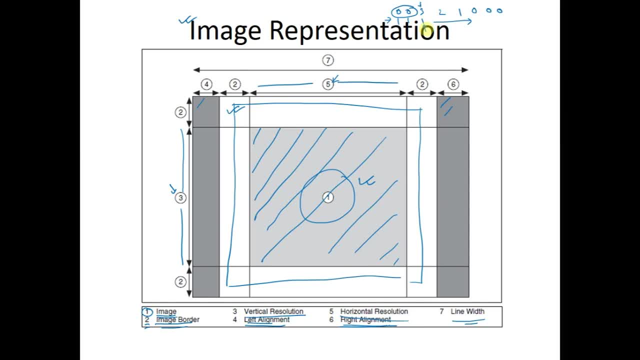 convolution, was there signal convolution? so in signal convolution, what you have done? so if you are having one signal- three, two, one, and this was your origin- and you have to convolve it with another signal, or say filter coefficients, say one, two, one, and this is the origin of that one, then what you do 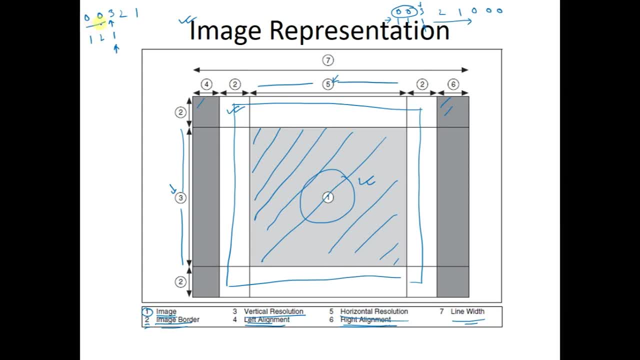 one multiplied by zero, two multiplied by zero because there are no values over here. so that was this: signal was padded with zeros and again, when we want to get the other outputs and we slide this values over here, we will be needing again padding on the right hand side also, right. 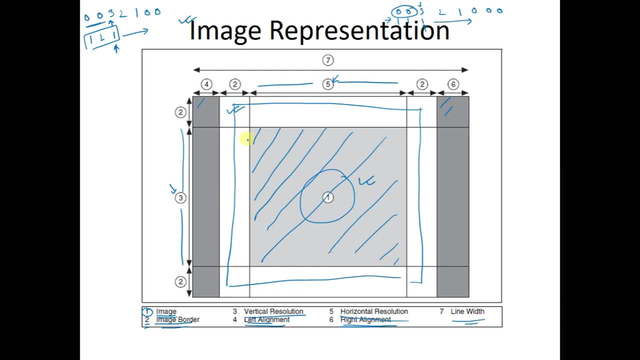 now, when we are talking about the images, it is a 2d signal, so the filter coefficients over here will also be a 2d element. okay, say, the simplest most is 3 by 3 matrix. okay, now how the thing happens over here. we had to match the origin. 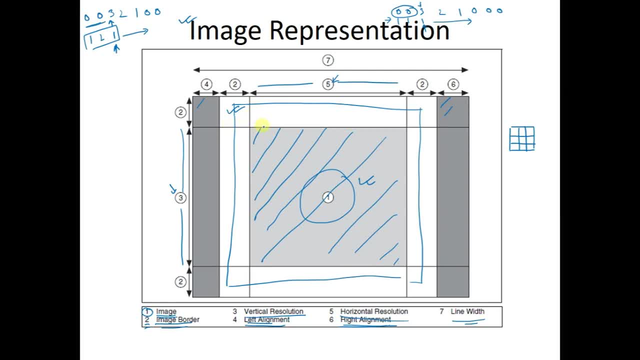 okay, now the origin of the image is here: zero, zero. are you getting my point? i told you just in the previous slide, origin is at this top, most left part, right. but when we are designing the filter, the origin is the central pixel. so you have to match the origin pixels. 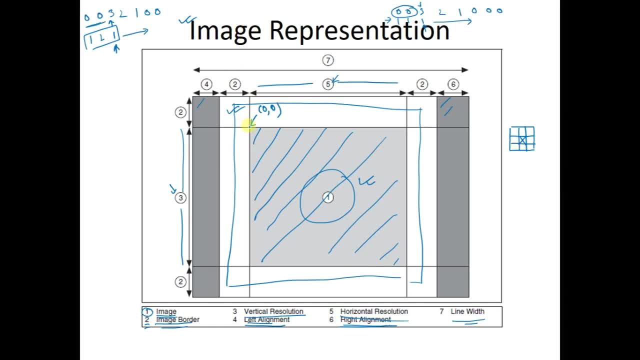 okay, so when we are trying to match the origin pixels. so if you try to do this, this is the origin pixel, but if you do not create the border, which is basically contemporary to the zero padding, you will not get any output for getting y zero in this case. you needed these values. 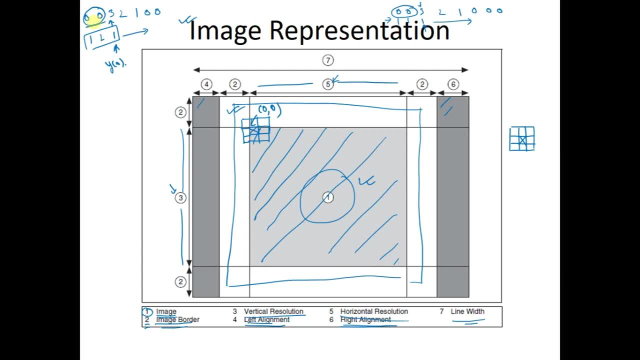 if these values are not there, you will not be able to calculate. the same thing is here also: if you do not create border and if you do not have the border values, how will you get the value of the origin of the pixel, the origin of the origin pixel of the image, right? it's not possible, so we need to. 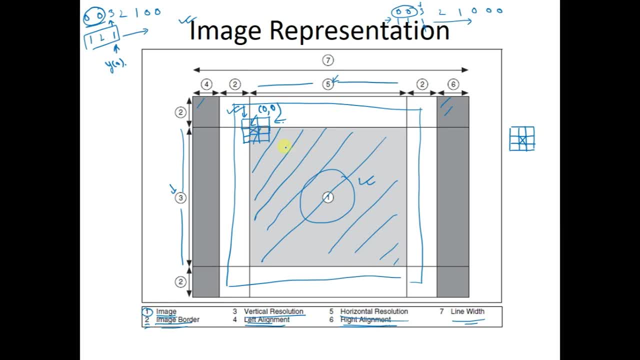 have a border. okay, if we are in between anywhere, doesn't matter, we will get all the pixels. those will be covered of the filter provision, they will be covered, right, but especially the edge pixels. for the processing of the edge pixels we need the border, okay. okay, but if you talk about matrix convolution, 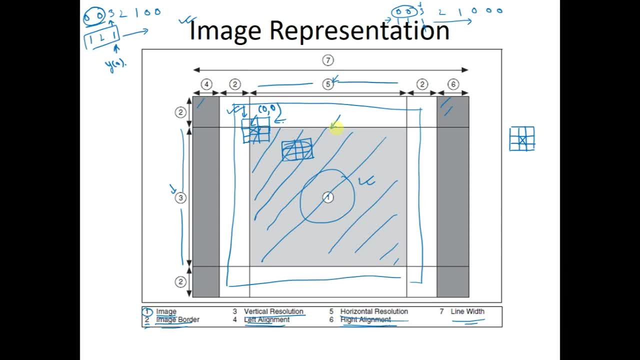 you do not need borders, just do the matrix convolution. this is one of the important difference between the matrix operation and the image processing operations. both are similar. you will find convolution correlation in the matrix operation also. you will find in the image processing also, image processing also. but there is a certain difference in this operation. 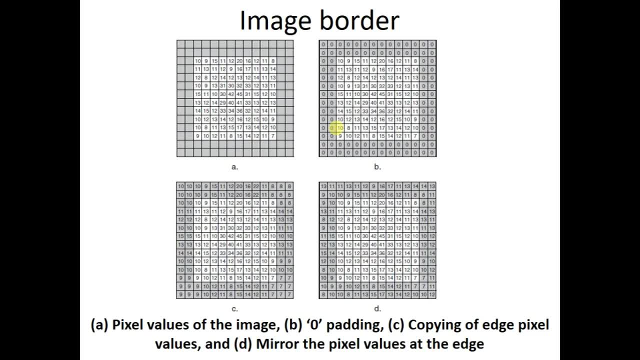 Now the important thing. so how to create the? now we have understood why we need border. Now the next question is how to create border. If it is a 3 by 3 filter matrix, then how many borders we need to create? We need to create a border of 1.. 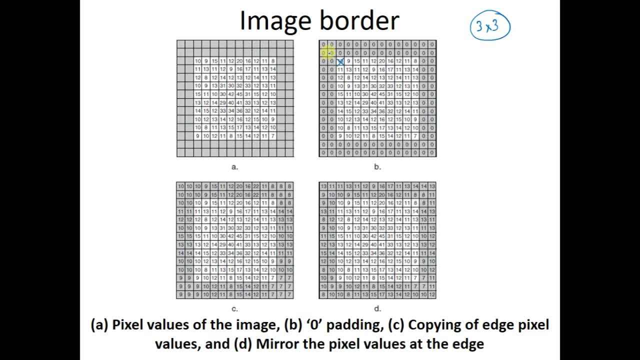 Why Suppose, this is the origin pixel, Right? So we need to create one line of border, even if we move this one. So when you are processing this pixel, we need border Only one border. Okay, If we have to process the image using a 5 by 5 filter, then we have to create two borders. 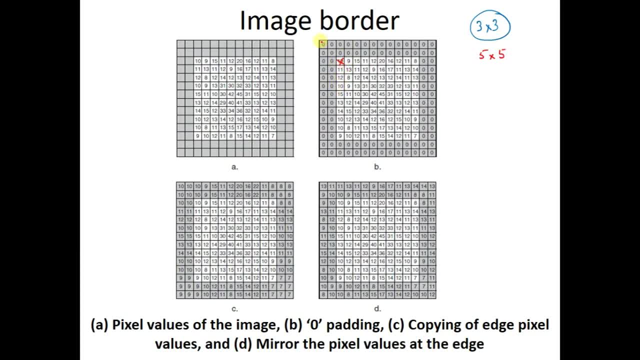 How come? This is the center. 5 by 5, right, If I want to go for this one. 2, the same thing. So we need at least 2 layers of borders, right? So if I have to generalize this, so, 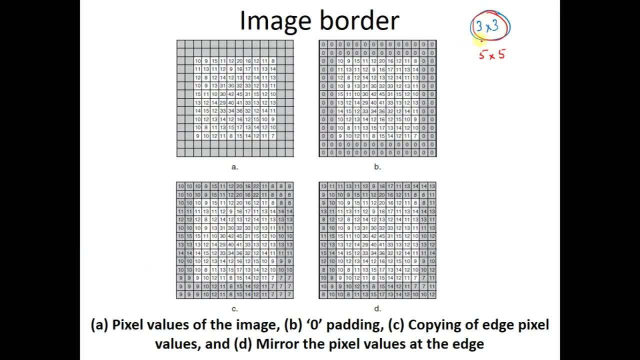 it becomes. whatever is this kernel size? we also call it as the kernel size of the filter: 3 by 3 or 5 by 5.. So n, which is basically the number of the layers of border, is equal to say k minus 1 divided by 2, where k is the generalized form of k by k, kernel k by. 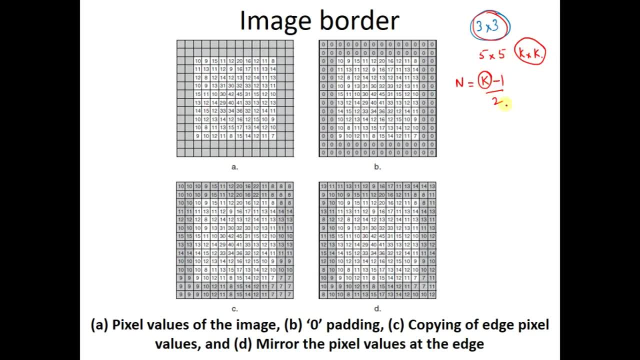 k kernel size. okay. So k minus 1 divided by 2.. So 3 minus 1 divided by 2. 2 is 1, so we need 1 layer of border. okay If it is 5 by 5, 2 layers of border If it. 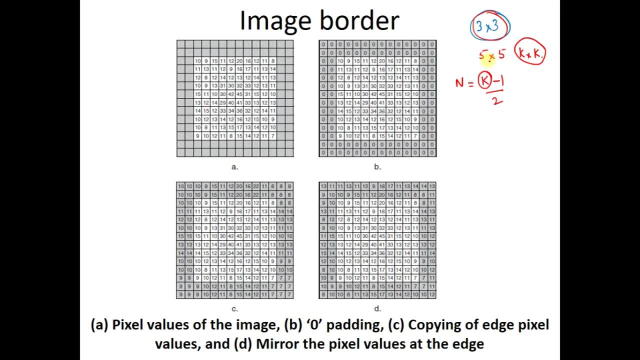 is 7 by 7, 3 layers of border, okay, And so on. Now the simplest part is 0 padding. You pad the border with 0. That's it And you are good to go. okay, Just like what you did in the one-day signal. You just put 0s and you do it. But there are 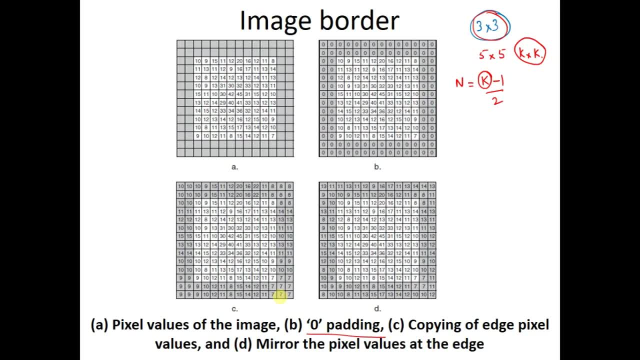 certain problems over here. What is the problem, If you see, this is the image 0 means completely dark, And when you are creating the border and when you are trying to create a filter, so what it will do It is looking at a when it is crossing this border, it is looking at a edge, Okay, So 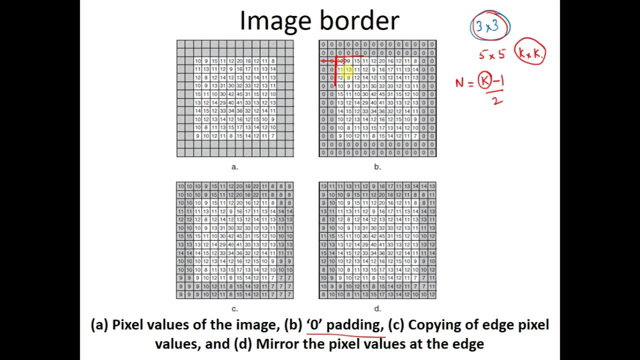 if you do high pass filtering, this edge values will be detected as the. this will be acting as the edge. this border pixel values- This will be acting as the edges And it would be detected as the edge. Okay, contour of the image, But that is not true. That is not true. You are not having a what? 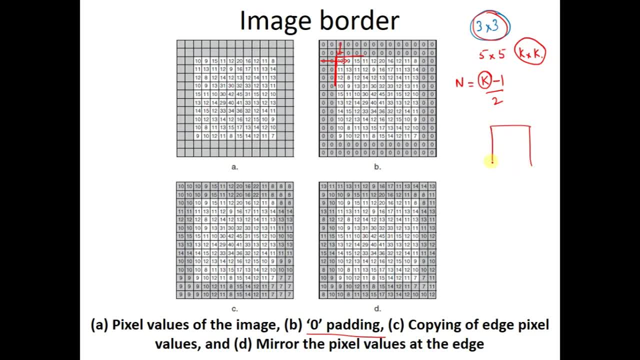 is an edge, Suppose you are having an object over here. So this is the background. So whenever you are moving from the background to the foreground, background will be darker, foreground will be brighter, usually, Or even when you move from foreground to background. there. 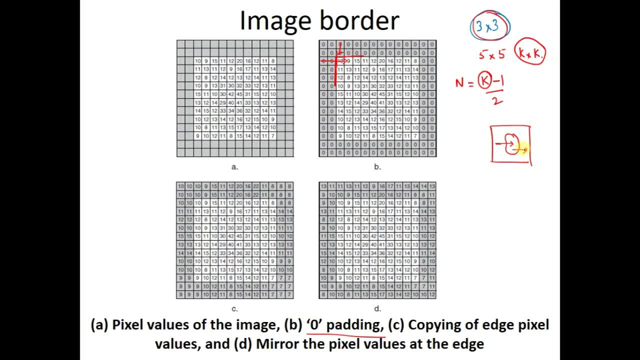 is a sharp change in the intensity levels, And they are. when there is a sharp change, they are high frequency components, right. So there will be an artificial creation of an high frequency component At the edges. So you will be getting a fallacious reading. Okay, You will be getting a fallacious. 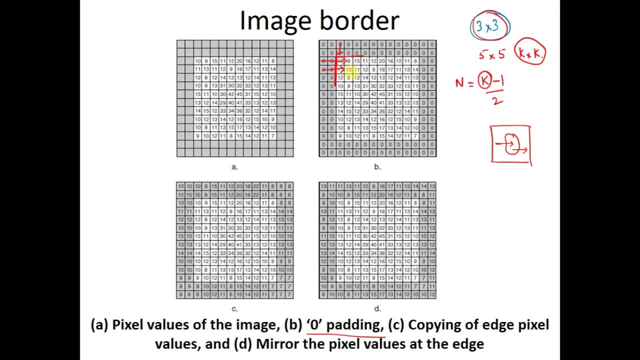 reading. So because of this, we would not consider 0 by 0 padding, though it is one of the simplest methods, But you will find that it creates a lot of noises in the, especially at the edges. it creates noises Okay. So usually we avoid 0 padding. 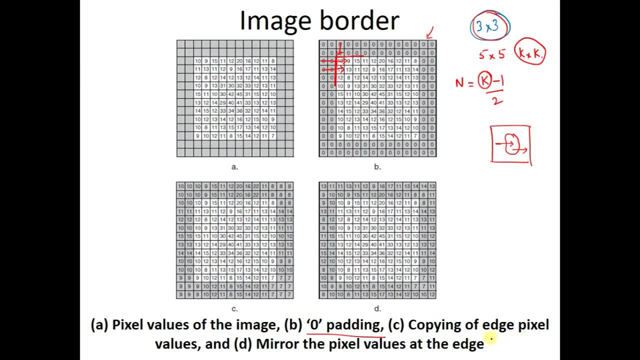 So now how to solve this. First one is copying of edge pixels. Okay, Now this example. it is basically for 5 by 5 kernel, But for 3 by 3 kernel. you just consider that these values are not there, These second row values. So, copying the edge pixels, this is the 10.. 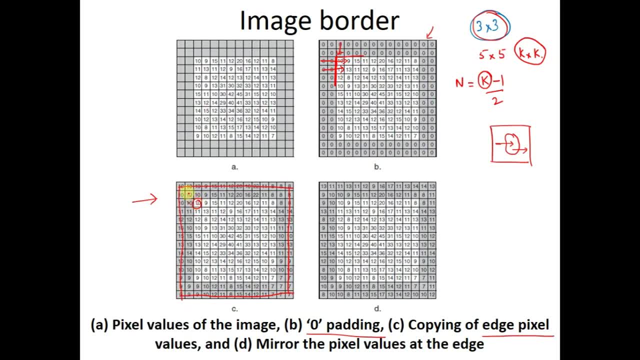 This is getting copied. This is getting copied. this is getting copied. this 9: it is getting copied. this 15: it is getting copied. 11: it is getting copied. Similarly, if you consider over here, see the first layer over here: 10, 10,, 10, 10,. 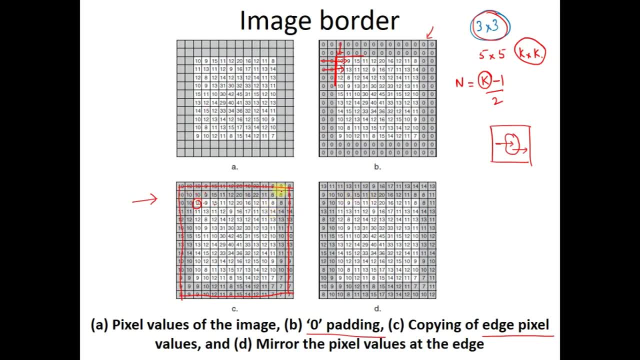 9,, 15,, 11,. these are matching in the copying and in the mirroring of the pixel values at the edges. But the difference comes if you need to create two layers of border. what is happening if you look over here? this value is 10.. 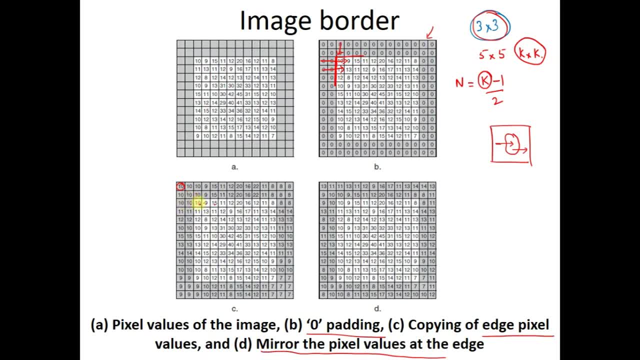 So we are copying These values, these edge values, so these values are getting copied. This 9, it is again being copied over here, But if you look over here, we have created this 10.. Now, when we are talking about mirroring, this is the mirror point: 10,, 10,, 13,, 13.. 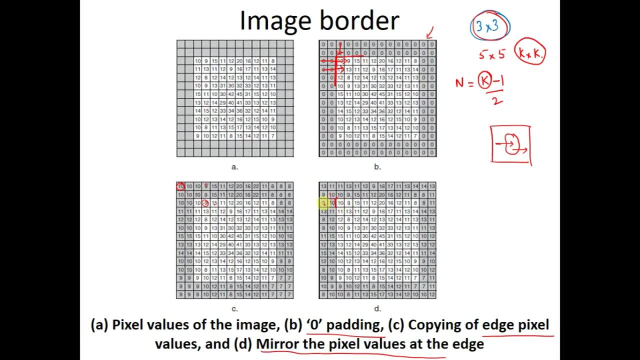 Then, if you consider this as the mirror point: 10, 10,, 9, 9.. Similarly, if you consider over here, 10, 10,, 11, 11.. Now you would say: so what about this one, what about this one and this one? how you. 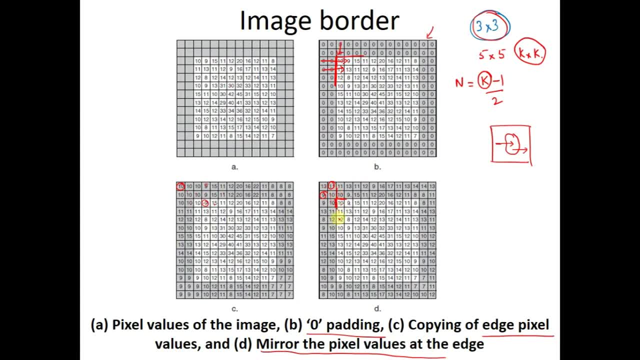 are getting. If you consider this: you have got 10 over here, you have got 10 from here. you have got 10 from here, then 9 from here. when you are mirroring, Then this: if you consider this as the symmetrical line, then this 9 will be replicated over. 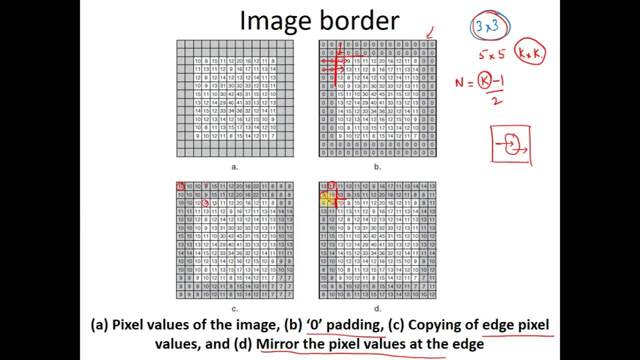 here. Similarly, over here also, this is a 10, then over here we are having 11, this 11 is getting replicated over here, But in this case, see, all this whole area is 10, because we have just copied the edge. 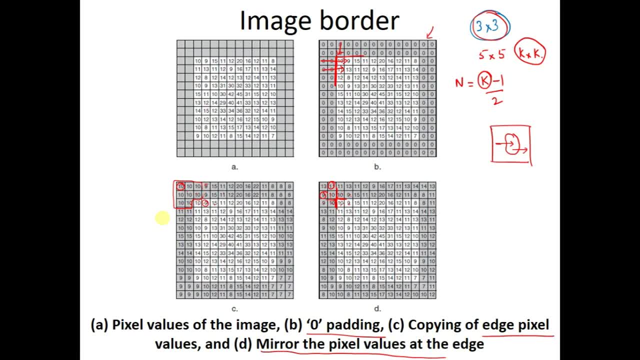 pixel value. If you are having, you have to create only one border. there will be no difference between copying of the edge pixel values- Okay- And then mirroring of the pixel values. But if you have to create two or more number of borders, then there will be a change. 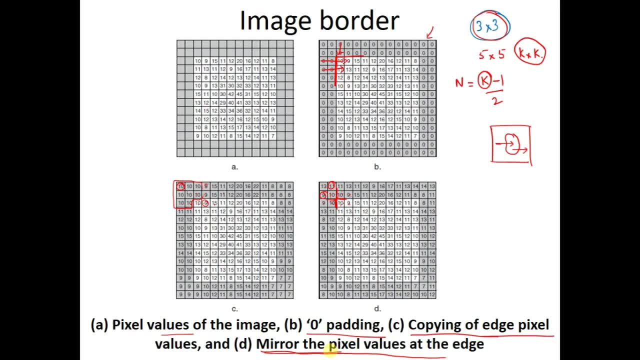 Okay, Sir. in the C, in the very last column, the value is repeated to 1 and 2.. Which one? 1 and 2.. Okay, But I will have to make a new one. Which one are you talking about? 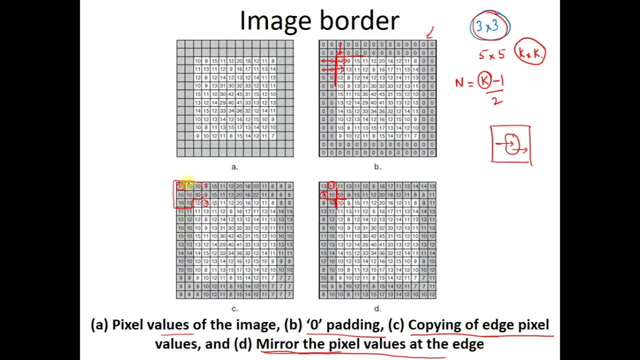 3rd row from top, 3rd row from top And 3rd column as the confidence. That is 1.. That is an error. This is 12.. This is a printing mistake. This should be 12.. 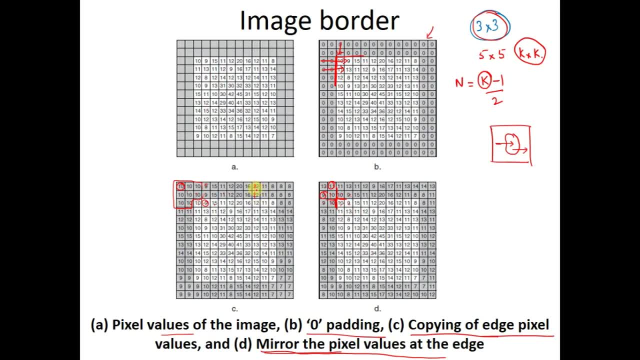 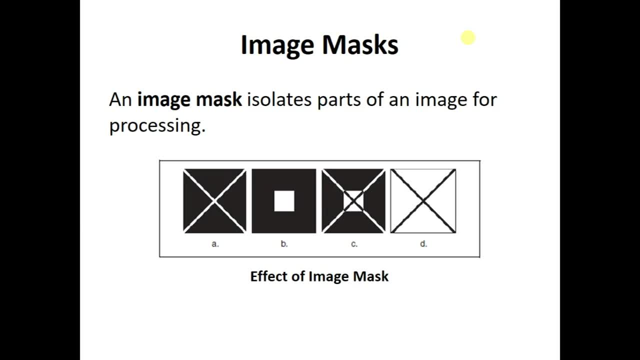 Thank you. Thank you, Prithip, So image mask, and image mask isolates parts of an image for processing. okay, Suppose you are having an image- this one- and then B is your mask, A is your image and B is your mask. okay, 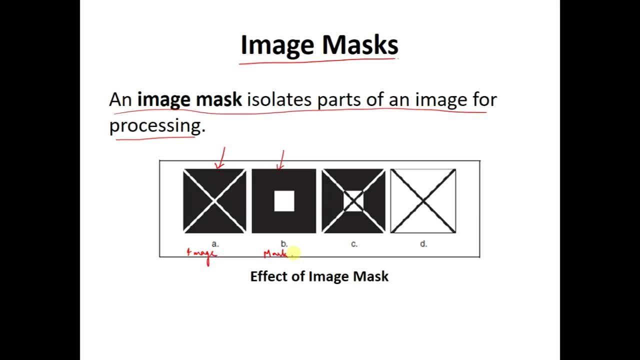 So if we apply an inversion- What you call inversion algorithm- on the image after we have applied the mask, then if you place the mask over here, Because if you superimpose these two, you will be getting a window, this white colored window, over here. 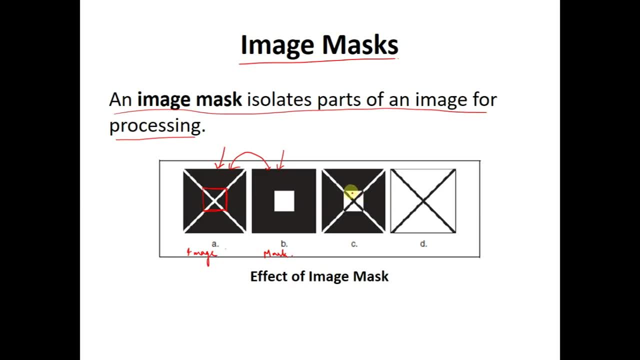 And when we apply the inversion, only see this box portion is getting Changed. If we are not using the mask, then what happens? The whole image changes, okay. So what image mask is doing? Image mask is allowing us to isolate a particular area within the image, okay. 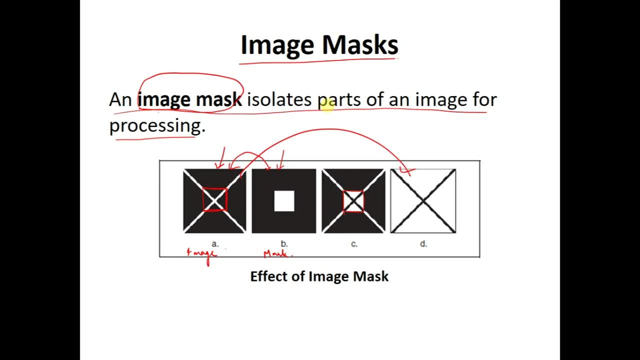 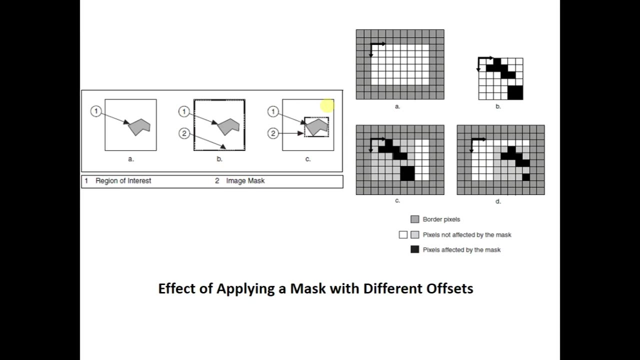 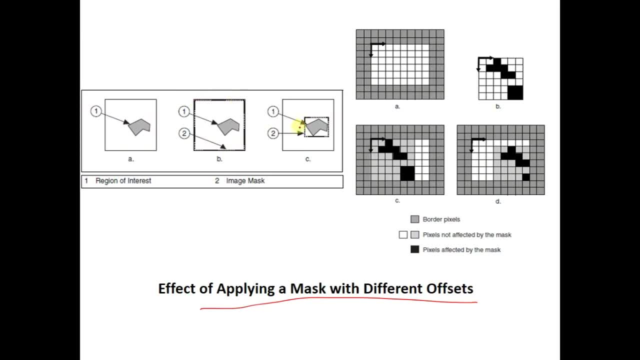 So it will. 2 is your whole mask. So then, if you want to find out this thing, So this is the region of interest and it is finding out the mask. So this is when the mask size and the image size are same, and this is when the mask and the region.